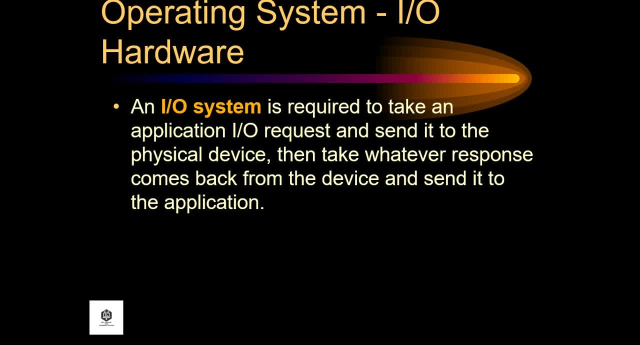 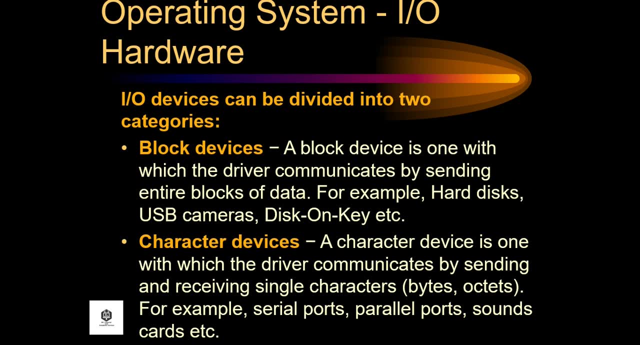 Then take whatever response comes back from the device and send it to the application. Input-output devices can be divided into two categories: Black devices- A black device is one with which the driver communicates by sending entire blocks of data, For example hard disk, USB cameras, and this on key. 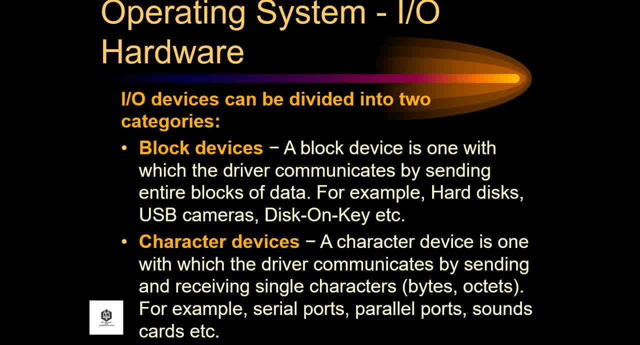 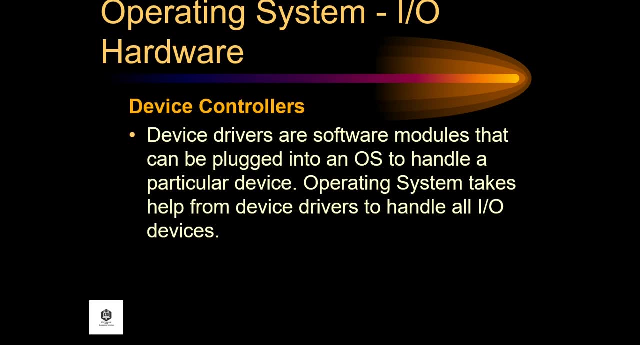 Next is the character devices. A character device is one with which the driver communicates by sending and receiving single characters, such as bytes or octets, For example serial ports, parallel ports, sounds cards, etc. Device controllers- Device drivers- are software modules that can be plugged into an OS to handle a particular device. 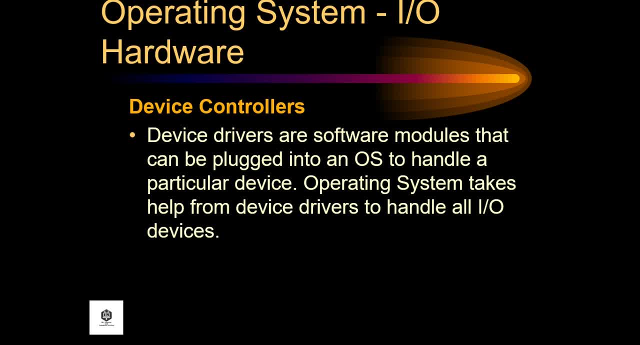 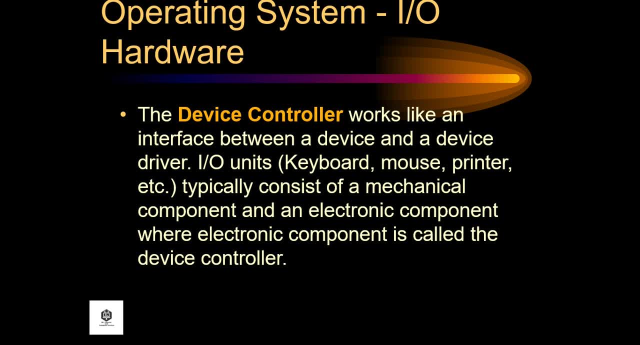 Operating system takes help from device drivers to handle all input-output devices. The device controller works like an interface between a device and a device driver. Input-output units, such as keyboard, mouse, printer, typically consist of a mechanical component and an electronic component, where electronic component is called the device controller. 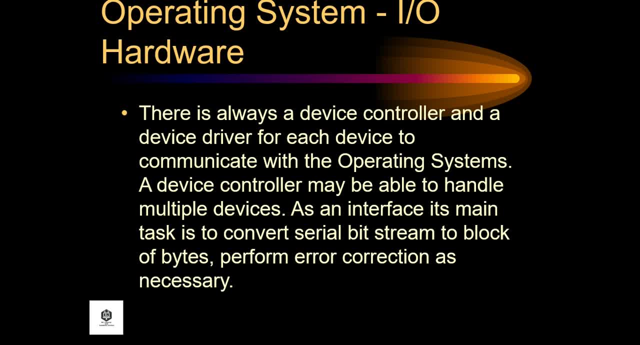 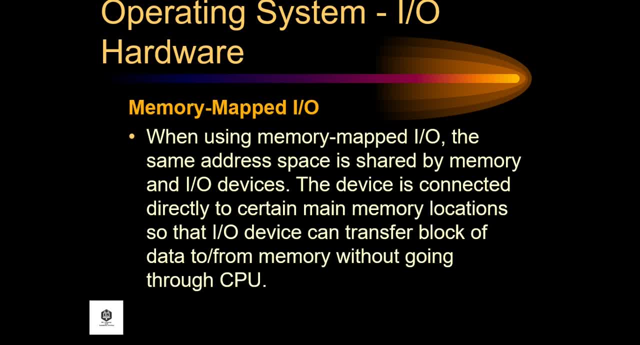 There is always a device controller and a device driver for each device to communicate with the operating system. Next is the MemoryMap® input-output function. When using MemoryMap® input-output, the same address space is shared by memory and input-output devices. 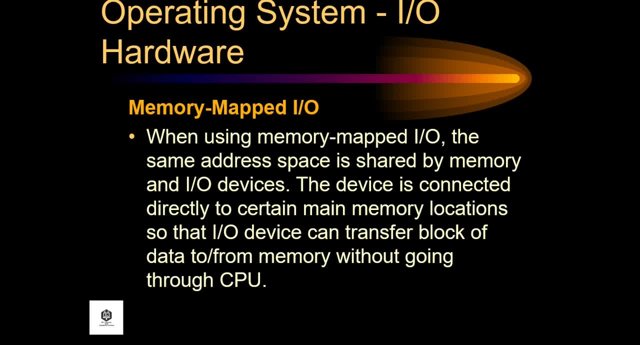 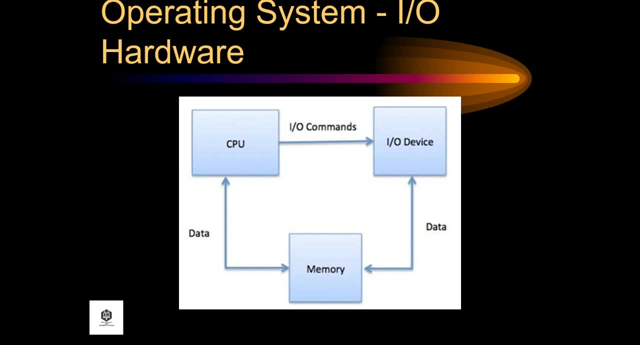 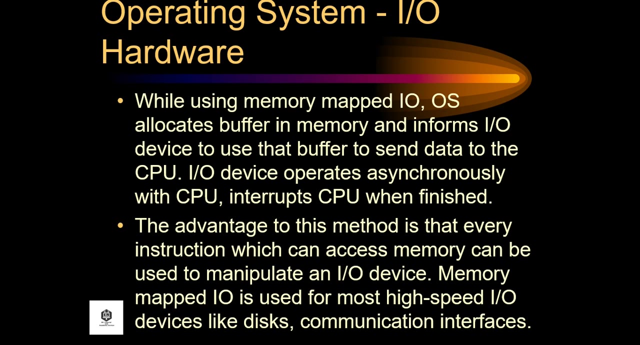 The device is connected directly to other main memory locations so that input-output device can transfer block of data to or from memory without going through CRMP Data Processor or CPU. This is the example image: While using memory map, input-output OS allocates buffer in memory and informs input-output. 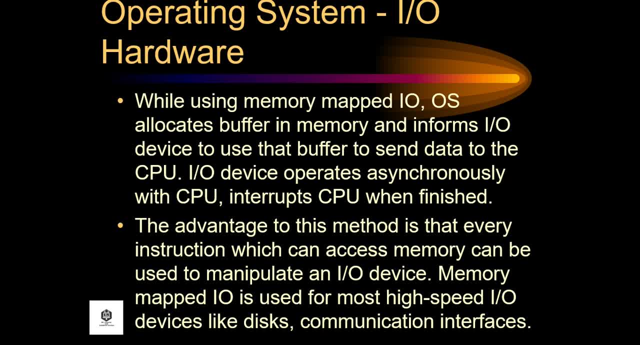 device to use that buffer to send data to the CPU. Input-output device operates asynchronously with CPU, interrupts CPU when finished. The advantage to this method is that every transaction which can access memory can be used to manipulate an input-output device. Memory map input-output is used for most high-speed input-output devices like disk communication. 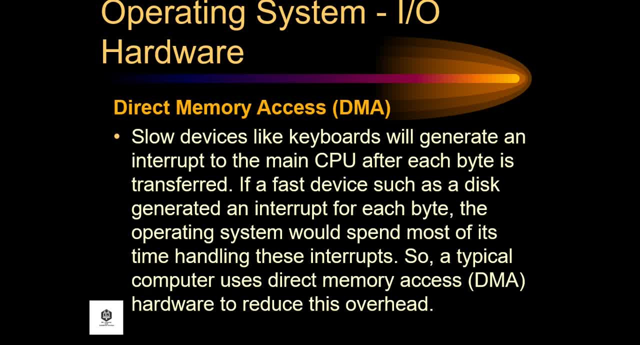 interfaces. The direct memory access or DMA. slow devices like keyboards will generate an interrupt to the main CPU after each byte is transferred. If a fast device, such as a disk, generated an interrupt for each byte, the memory map input-output device will generate an interrupt to the main CPU after each byte. 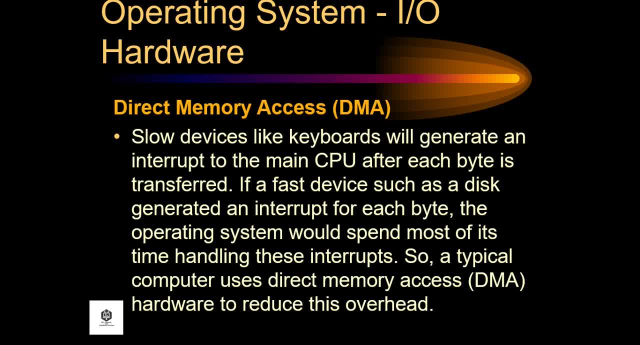 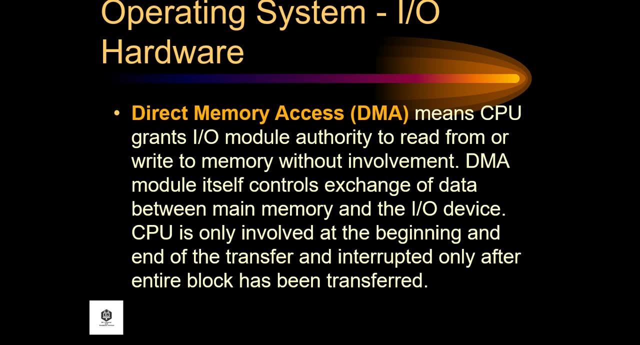 The operating system would spend most of its time handling these interrupts. so a typical computer uses direct memory access or DMA hardware to reduce this overhead. Also, the direct memory access or DMA means CPU grants input-output module authority to read from or write to memory without involvement. 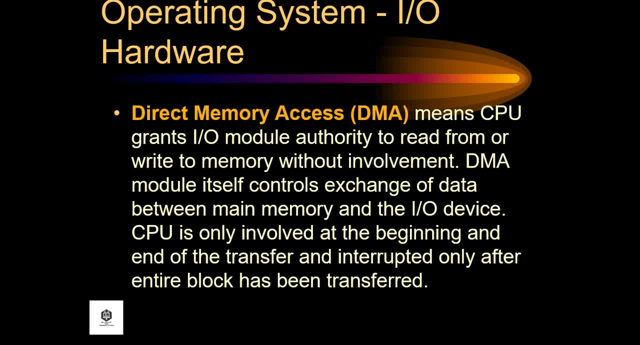 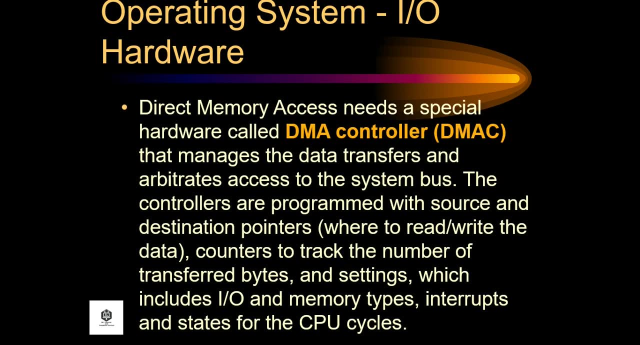 CPU is only involved at the beginning and end of the transfer and interrupted only after entire block has been transferred. Direct memory access needs a special hardware called DMA controller or DMACC that manages the data transfers and arbitrates access to the system bus. The controllers are programmed with source and destination parameters. 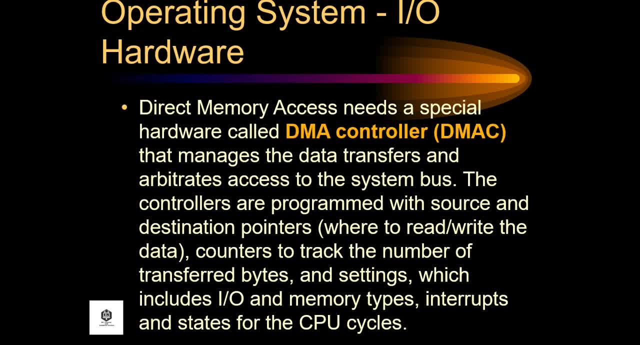 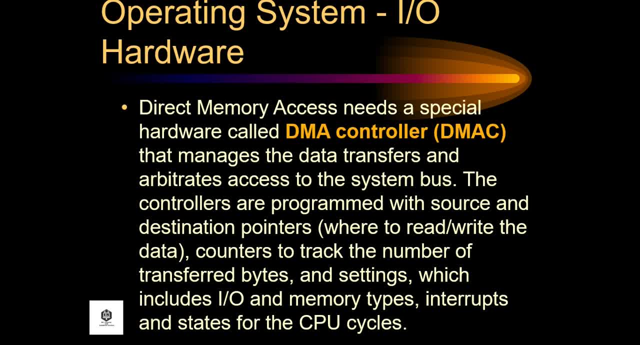 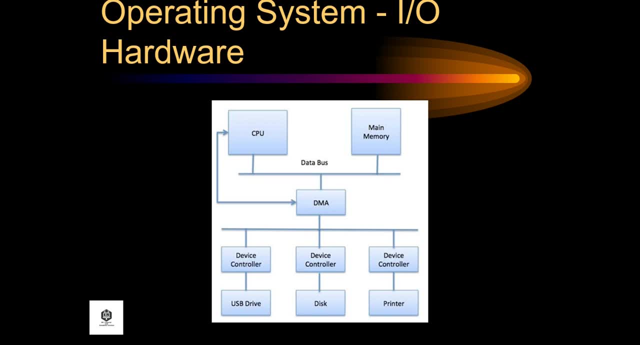 The Maria-Q, camaraderie and Iris insbesondere parameters. In this example here DMA is again called true Harbor DB, as it comes from samhiri model. In this example here DMA is called true Harbor DB, as it comes from samhiri model. 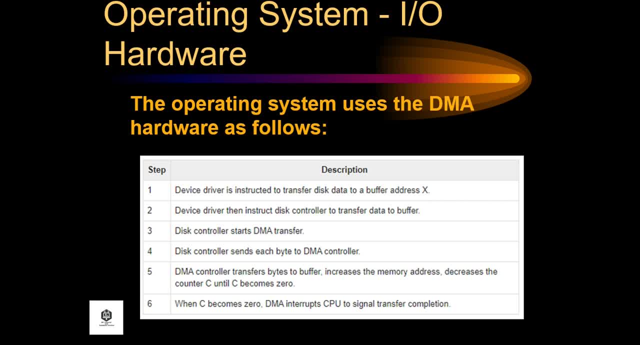 olsa P DataCom probe gamification required, DMA or Ramp Up пользовating software in advanced languages to自 boys iant 59p. I'll also talk whether everything works or perhaps helfen. Zakopane Ergofest as follows: device drivers is instructed to transfer this data to a buffer address. 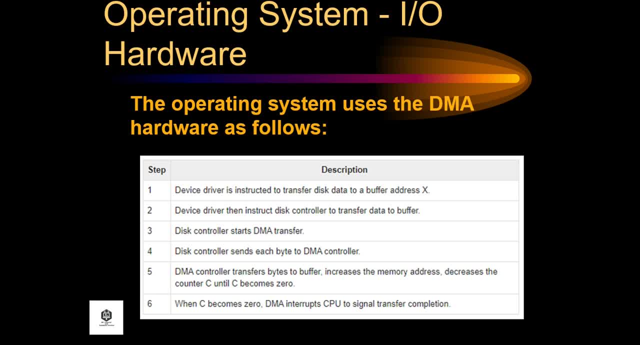 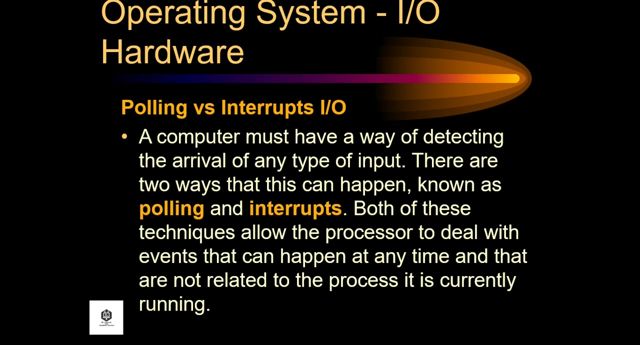 device driver then instructs this controller to transfer data to buffer. this controller starts DMA transfer. this controller sends each byte to DMA controller. DMA controller transfers bytes to buffer, increases the memory address, decreases the counter C and C become zero and once it becomes zero, DMA interrupts CPU. the signal transfer completion. 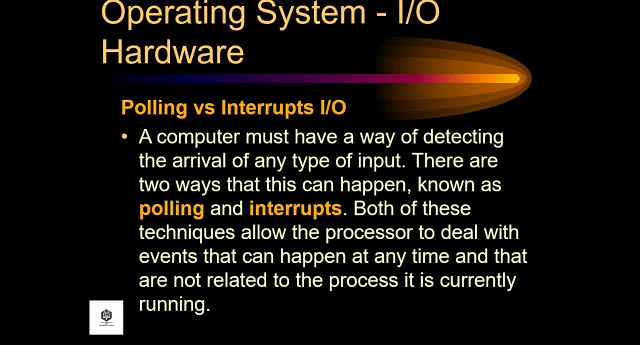 how about falling verses, interrupt input output? a computer must have a way of detecting the arrival of any in type of input. there are two ways that this can happen, known as falling and interrupts. this allow the processor to deal with events that can happen at any time and that are 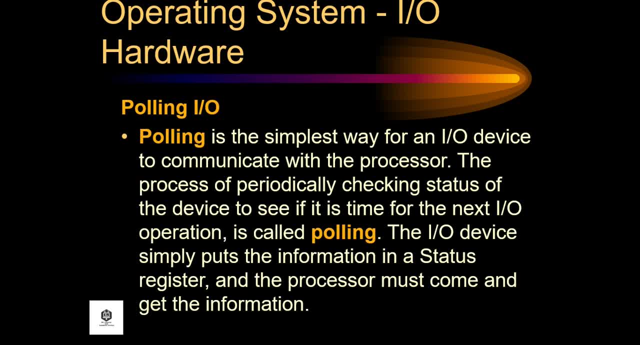 not related to the process it is currently running: The polling. input output. Polling is the simplest way for an input output device to communicate with the processor. The process of periodically checking status of the device to see if it is time for the next input output operation is called polling. 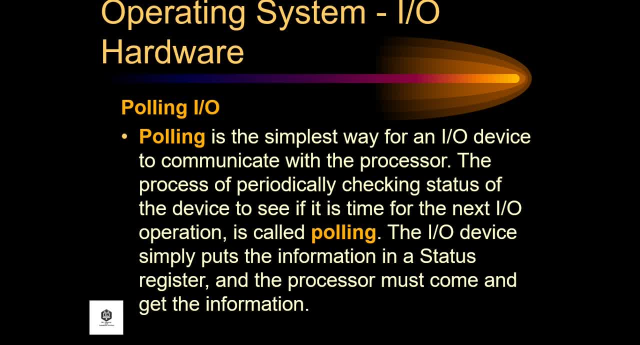 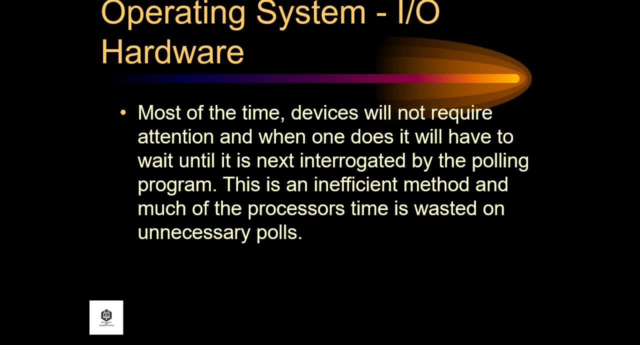 The input output device simply puts the information in a status register and the processor must come and get the information. Most of the time, devices will not require attention, and when one does, it will have to wait until it is next interrogated by the polling program. This is an inefficient method and much 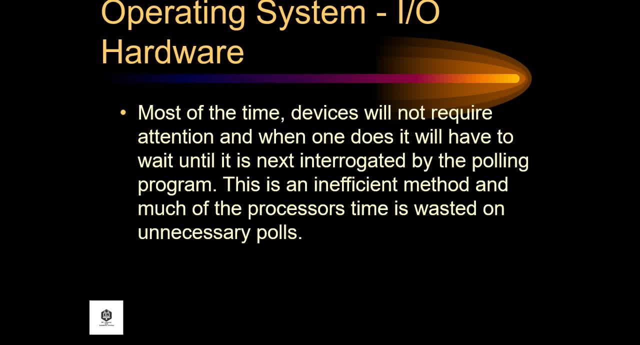 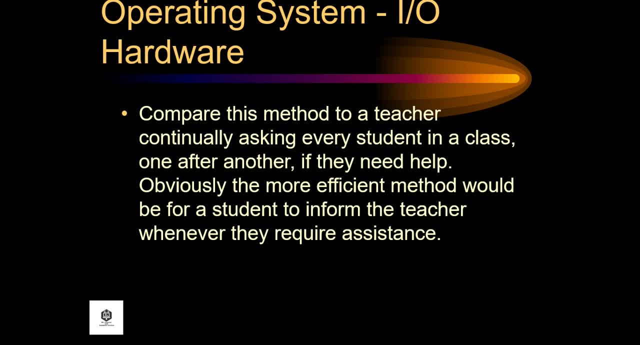 of the processor's time is wasted on unnecessary polls. Comparison: Compare this method to a teacher continually asking every student in a class, one after another, if they need help. Obviously, the more efficient method would be for a student to inform the teacher whenever they require assistance. 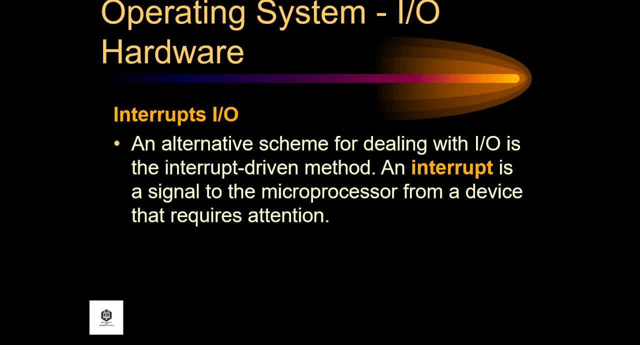 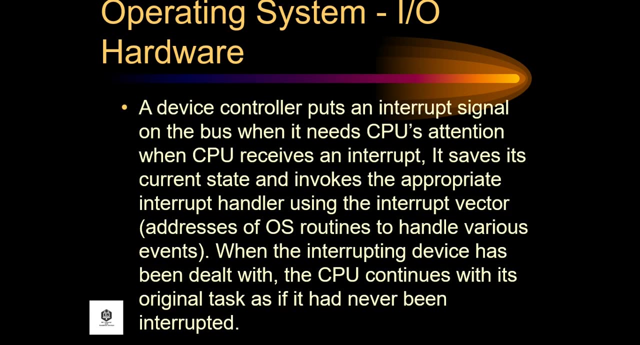 How about the interrupts input output? An alternative scheme for dealing with input output is the interrupt driven method. An interrupt is a signal to the microprocessor from a device that requires attention. A device controller puts an interrupt signal on the bus when it needs CPU's attention. when CPU receives an interrupt, It saves its current state and 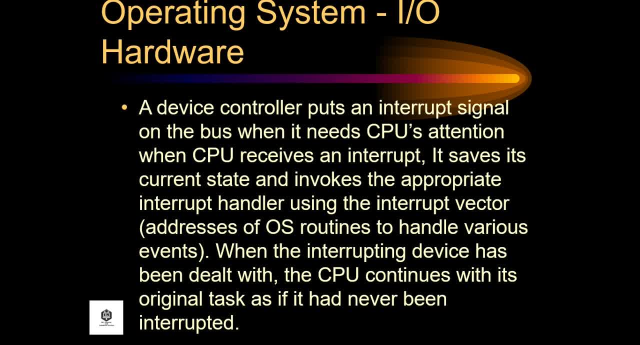 invokes the appropriate interrupt handler, using the interrupt vector addresses of OS routines to handle various events. When the interrupting device has been dealt with, the CPU continues with its original task, as if it had to do the same thing over and over again. It is not possible to 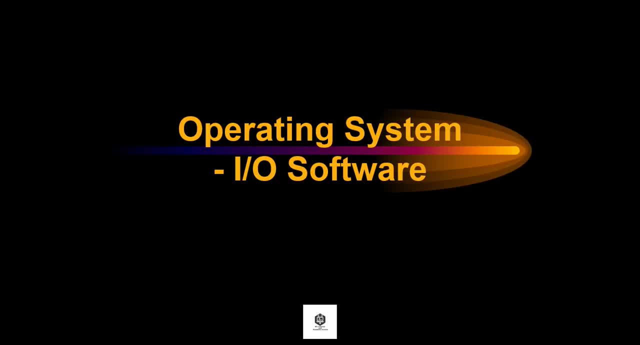 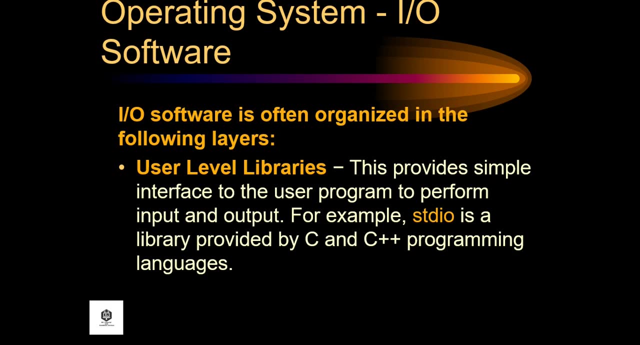 if it had never been interrupted. Let's proceed to the operating system in terms of input-output software. Input-output software is often organized in the following layers. First, user-level libraries. This provides simple interface to the user program to perform input and output. 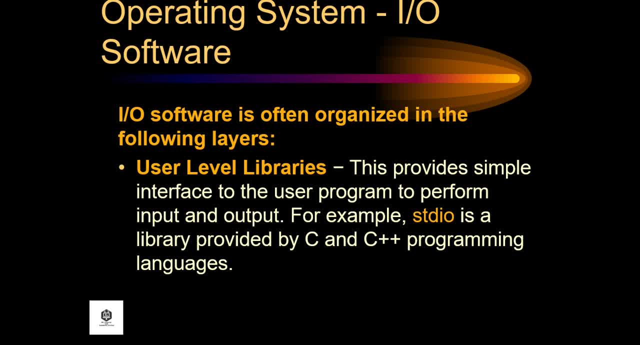 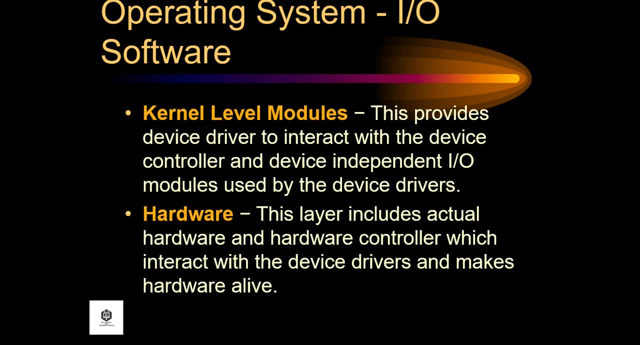 For example, STDIO is a library provided by C and C++ programming languages Kernel-level modules. This provides device driver to interact with the device controller and device-independent input-output modules used by the device drivers. Then the hardware: This layer includes actual hardware and hardware controller. 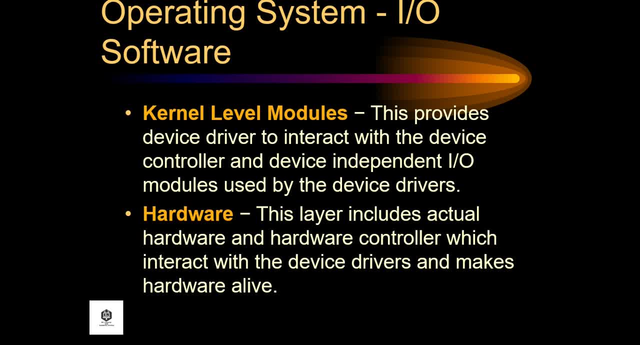 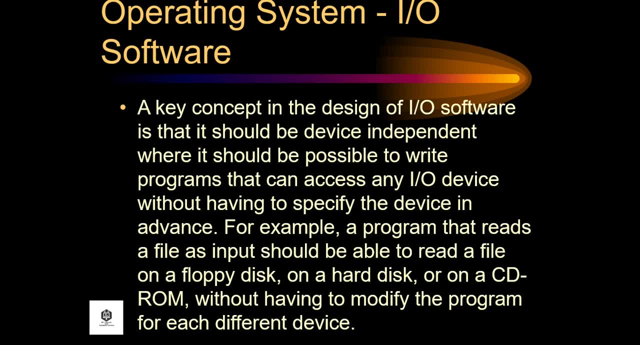 which interact with the device drivers and makes hardware alive. A key concept in the design of input-output software is that it should be device-independent, where it should be possible to write programs that can access any input-output device without having to specify the device in advance. 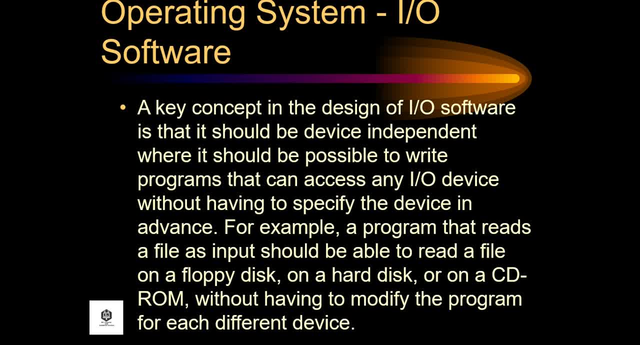 For example, a program that reads a file as input should be able to read a file on a ploppy disk, on a hard disk or on a CD-ROM without having to modify the program for each different device. So here is the sample image. 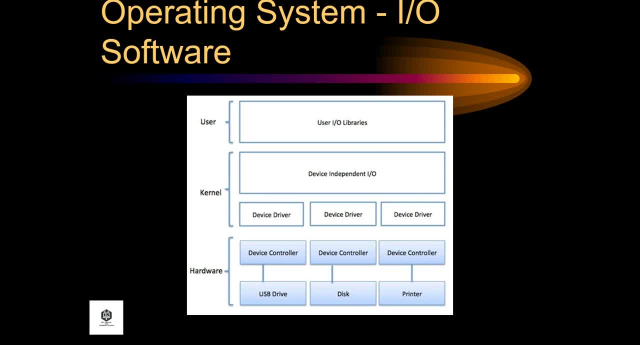 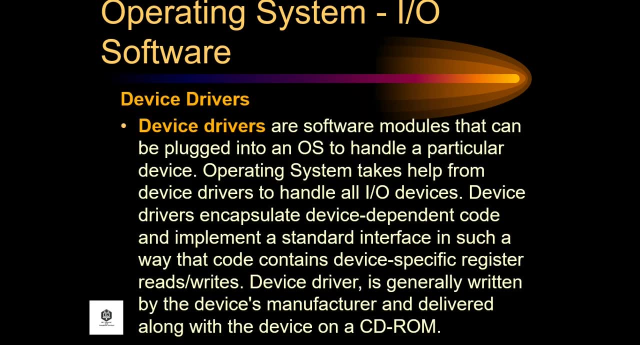 Here are the images of the user kernel and hardware. So the device drivers are software modules that can be plugged into an OS to handle a particular device. Operating system takes help from device drivers to handle all input-output devices. Device drivers encapsulate device-dependent 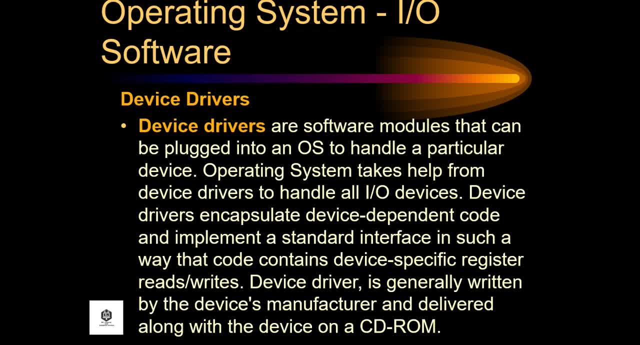 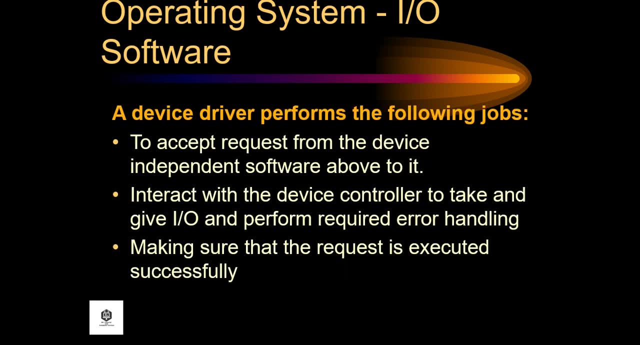 code and implement a standard interface in such a way that code contains device-specific register reads or writes. Device server is generally written by the device's manufacturer and delivered along with the device in a CD-ROM. A device driver prefers the following jobs: To accept requests from the device-independent software. 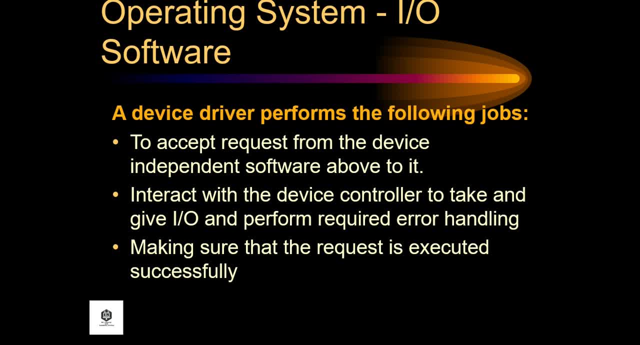 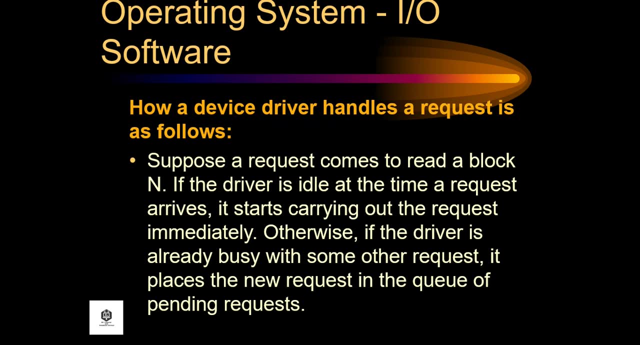 above to it, interact with the device controller to take and give input-output and perform required error handling, making sure that the request is executed successfully. How a device driver handles a request is as follows. Suppose a request comes to read a black N. 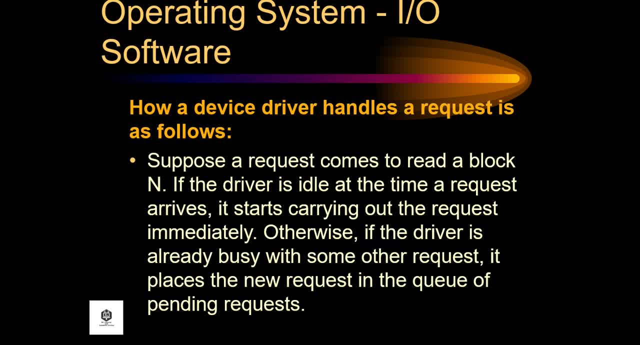 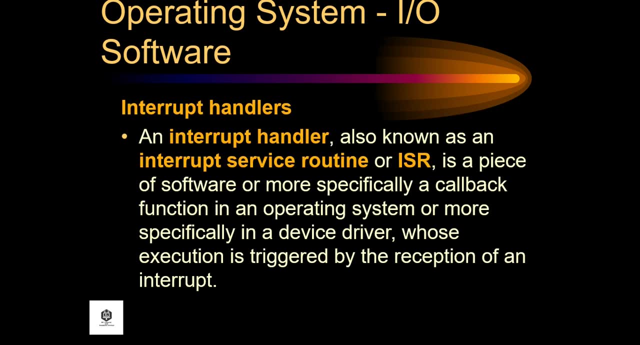 If the driver is idle at the time a request arrives, it starts carrying out the request immediately. Otherwise, if the driver is already busy with some other requests, it places the new request in the queue of pending requests. Interrupt handlers- An interrupt handler, also known as an interrupt service. 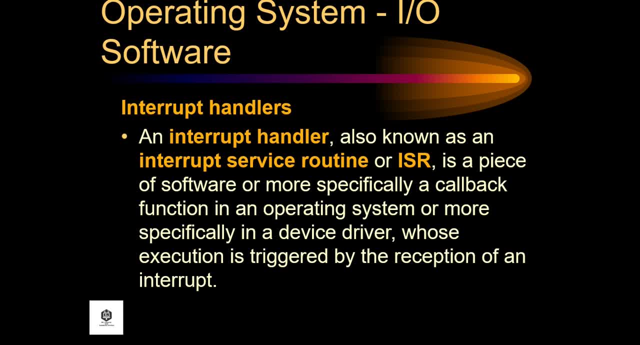 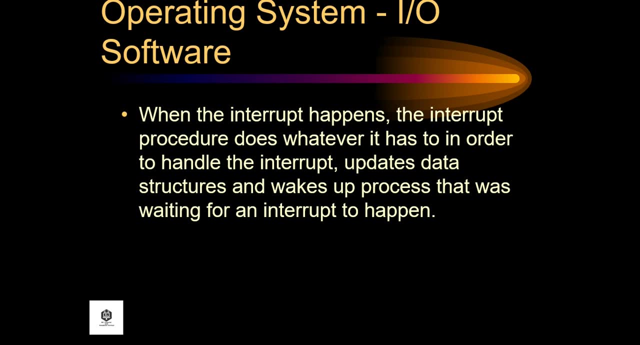 routine, or ISR, is a piece of software, or more specifically, a callback function in an operating system, or more specifically, in a device driver, whose execution is triggered by the reception of an interrupt. When the interrupt happens, the interruption action also occurs. 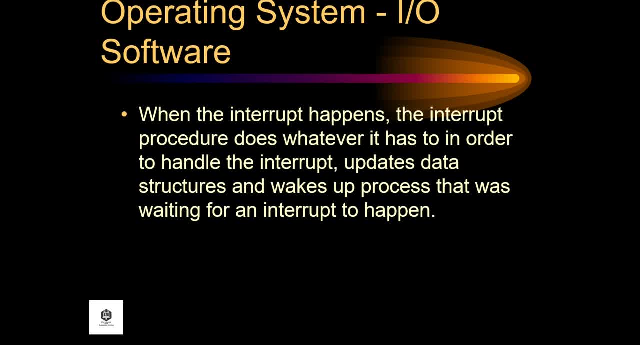 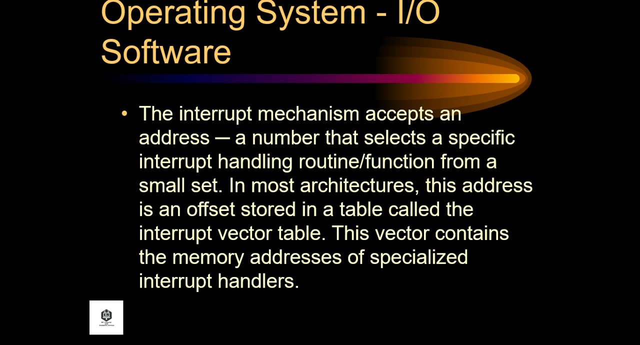 interrupt happens. the interrupt procedure does whatever it has to in order to handle the interrupt, updates data structures and wakes up process that was waiting for an interrupt to happen. The interrupt mechanism accepts an address, a number that selects a specific interrupt handling routine or function from a small set. In most architectures, this address is an offset. 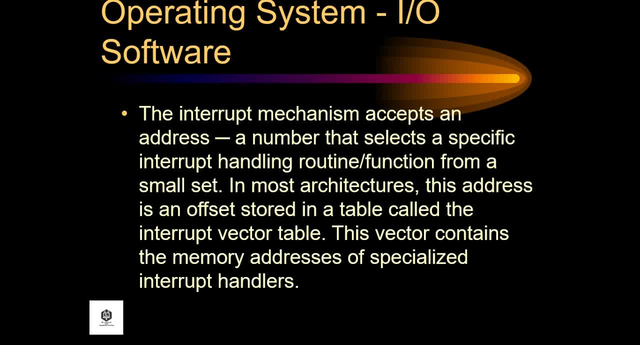 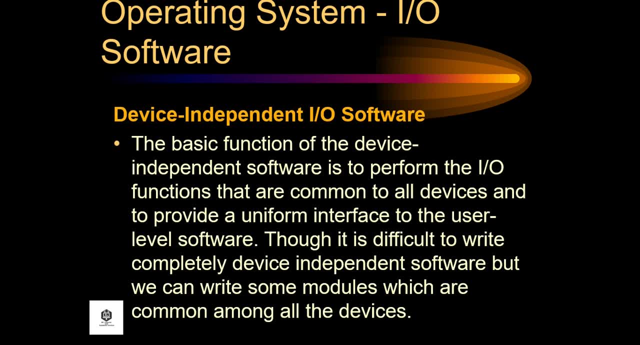 stored in a table called the interrupt vector table. This vector contains the memory addresses of specialized interrupt handlers. Next is the device-independent input-output software. The basic function of the device-independent software is to perform the input-output functions that are common to all devices and to provide a uniform interface to the user-level software. 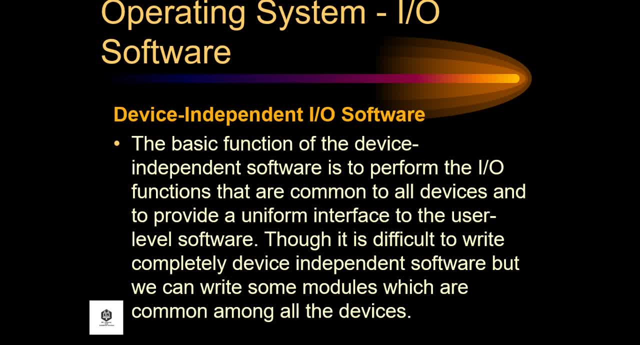 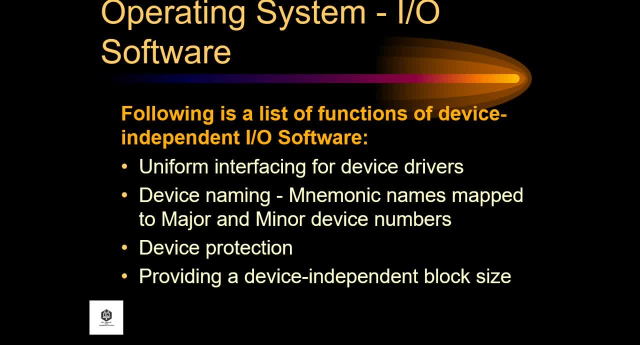 Though it is difficult to write the code, the interface is very easy to use, Completely device-independent software, but we can write some modules which are common among all the devices. Following is a list of functions of device-independent input-output software: Uniform interfacing for device drivers. device naming. 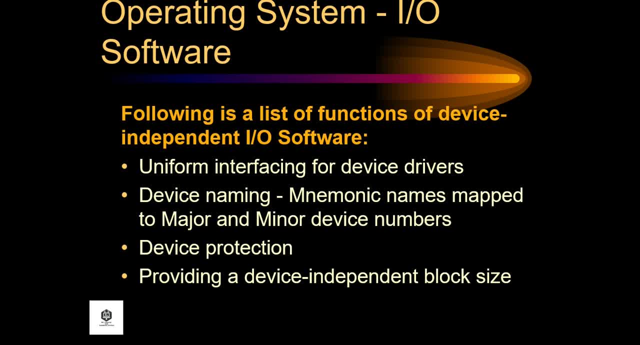 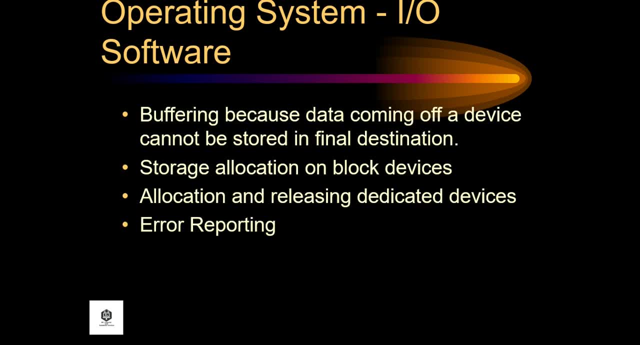 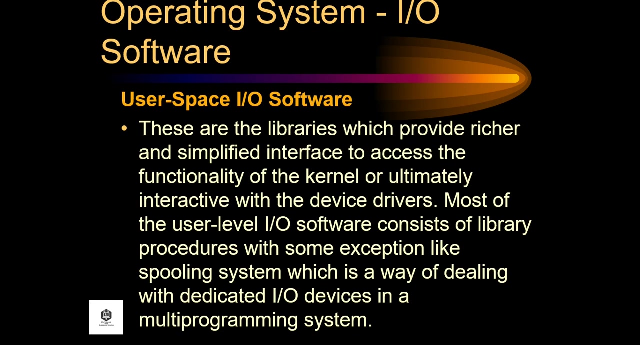 mnemonic names mapped to major and minor device numbers. device protection providing a device-independent block size. buffering, because data coming off a device cannot be stored in final destination storage. allocation on block devices. allocation and releasing dedicated devices and error reporting. The user space input-output software. These are the libraries which provide richer and simplified. 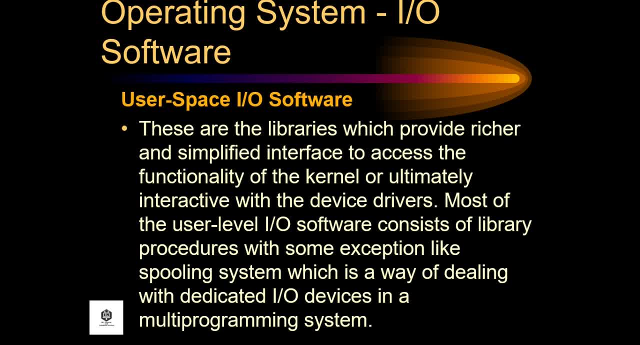 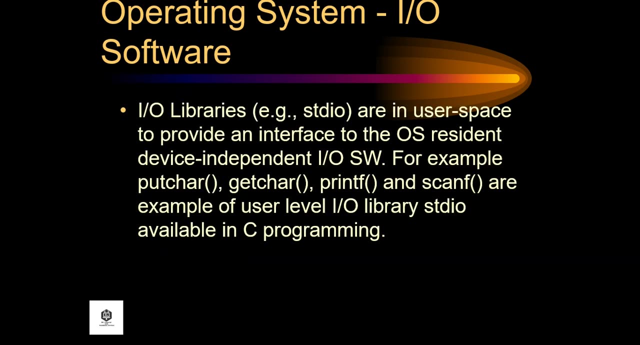 interface to access the functionality of the kernel and ultimately interact with the device drivers. Most of the user-level input-output software consists of library procedures, with some exception, like spooling system, which is a way of dealing with dedicated input-output devices in a multi-programming system. 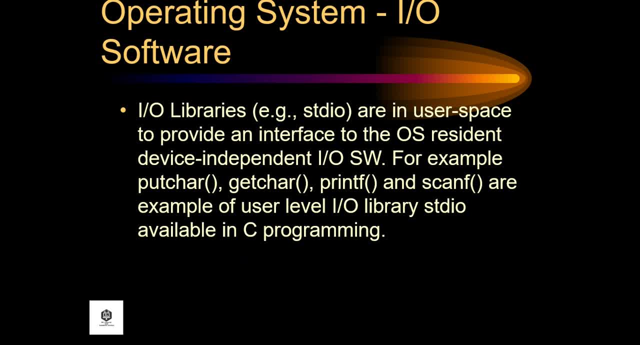 Input-output libraries such as STDIO are in user space to provide an interface to the OS resident device independently. It is only here that we can provide it書Just because of the number of hours it is required to dialed to find it. input-output software, for example PutCart, GetCart, PrintF and ScanF are examples of. 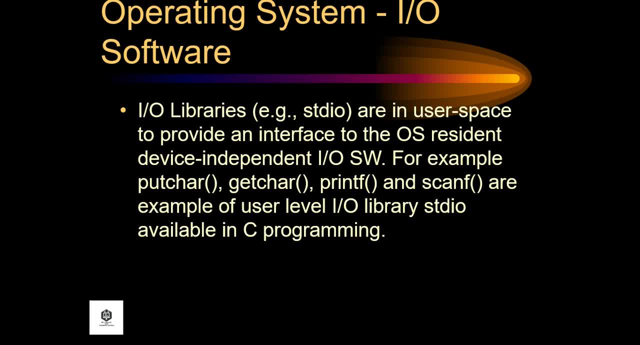 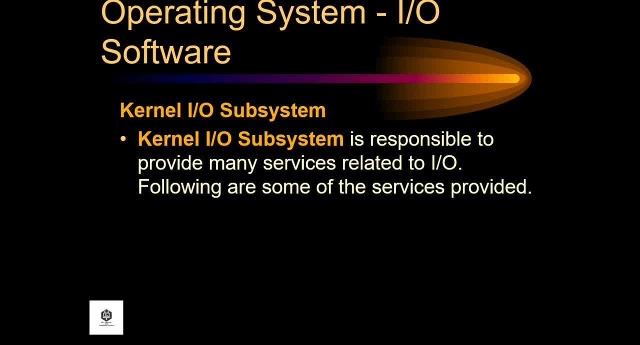 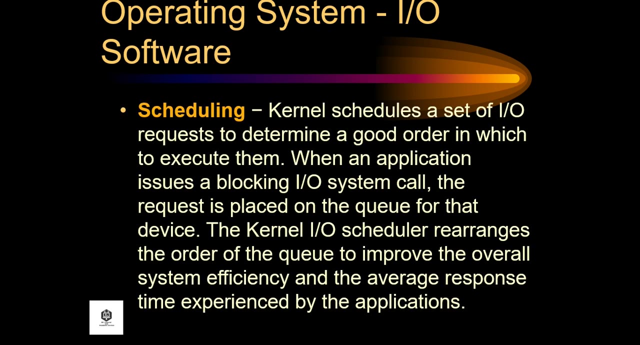 user-level input-output libraries- STDIO- available in C programming. Next is the Kernel Input-Output Subsystem. Kernel Input-Output Subsystem is responsible to provide many services related to input-output. Following are some of the services provided. First is the Scheduling. 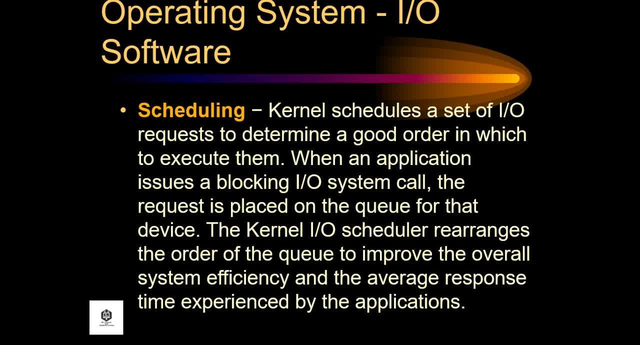 Kernel schedules a set of input-output requests to determine a good order in which to execute them. When an application issues a blocking input-output system call, the request is placed on the queue for that device. The Kernel Input-Output Scheduler rearranges the order of the queue to improve the overall system efficiency.